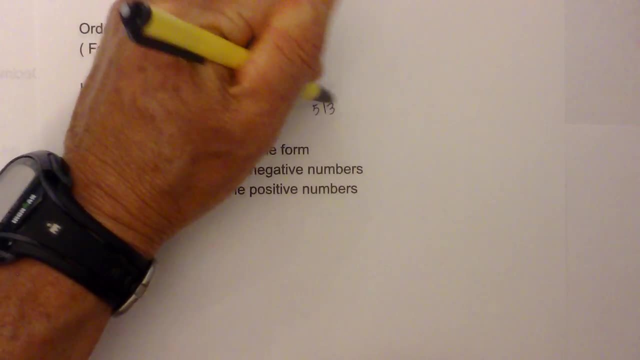 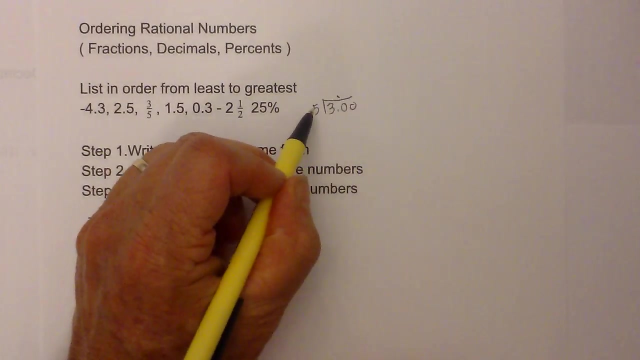 denominator. So I'm going to 3 here. divide by 5.. I'm going to put a decimal there. I'm going to make sure I put the decimal right on top. 5 goes into 3 zero times, but 5 goes into 36.. So it. 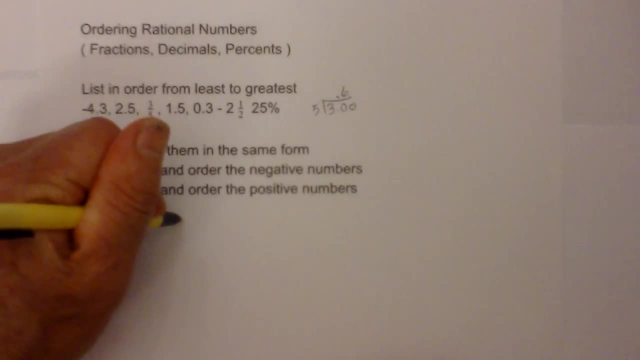 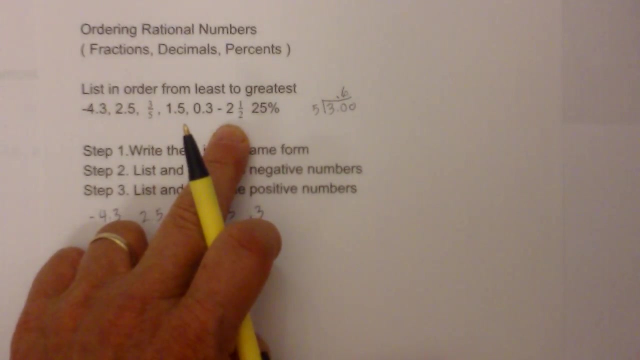 becomes 0.6.. So 3 fifths is 0.6.. I'm going to write 0.6.. Then I have 1.5 and then 0.3.. And how about negative 2.5?? Now I'm going to convert it to a mixed fraction and, excuse me, an improper fraction, and then 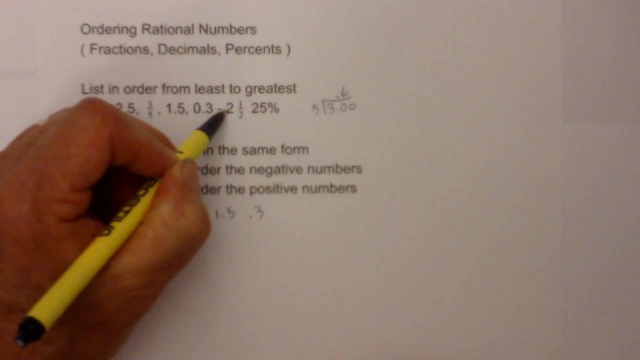 convert that to a decimal, So 2 times 2 is 4 plus 1 is 5.. And it'd be 5 over 2.. And then to convert this to a decimal, again, divide the numerator by the denominator, So it'll be 5. 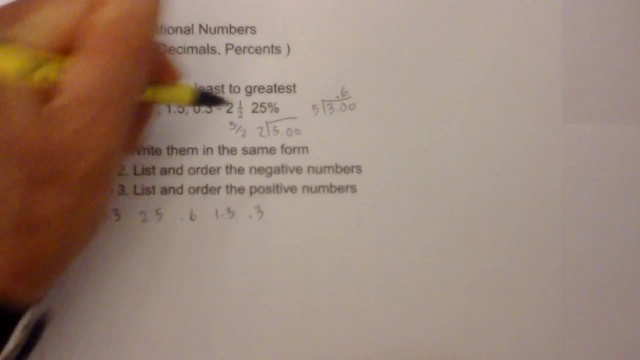 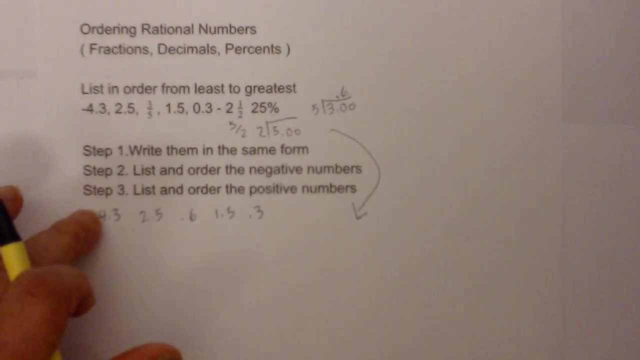 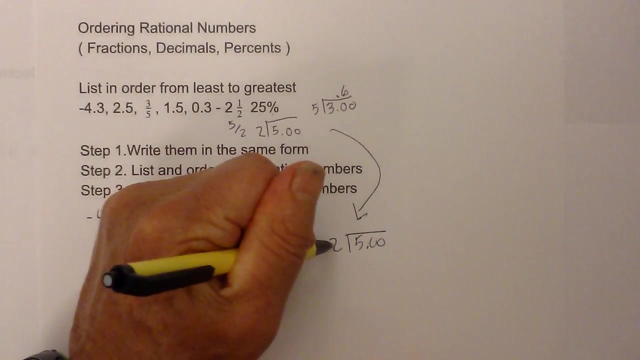 divided by 2.. Remember to move the decimal. 2 goes into 5 two times. I'm going to move this down right here. It's a little messy. Okay, So I have 5 divided by 2.. Okay, Let's see it. Yes, I still have it on. Make sure to put the decimal there. 2 goes into 5 two. 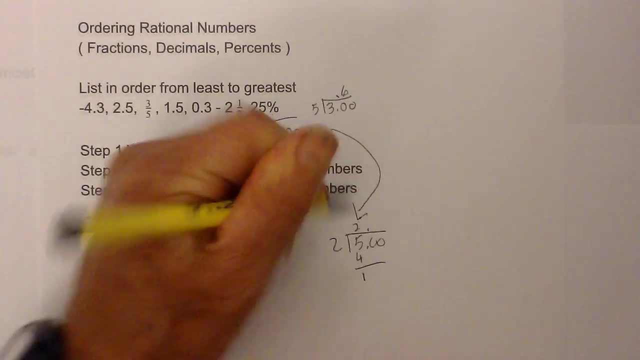 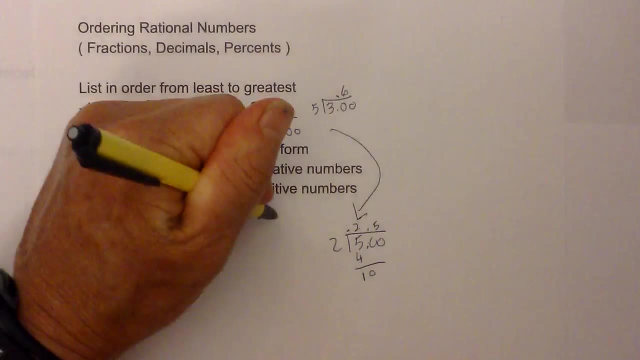 times 2 times 2 is 4.. Bring down the 1. 2 goes into 10, five times, So it becomes negative 2.5.. So now I have negative 2.5. And then for 25%. 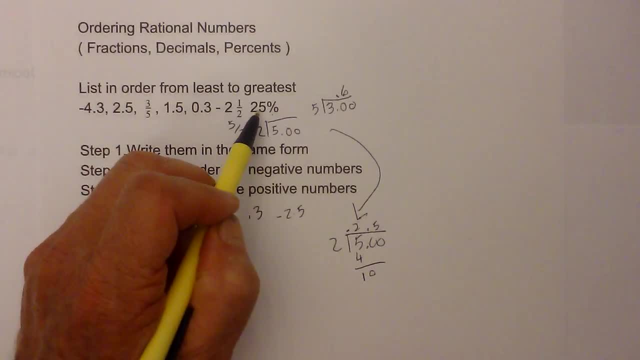 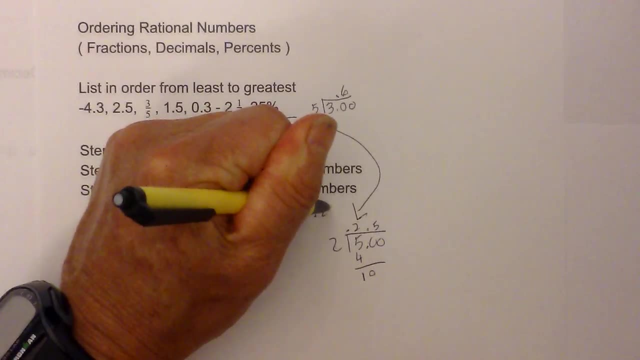 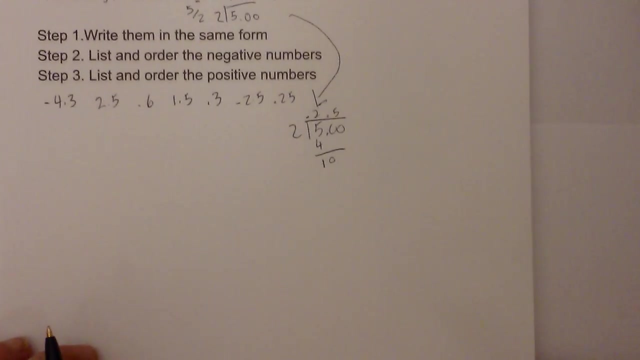 to change a percent to a decimal. you divide by 100. Or you can just move the decimal two places to the left So that becomes 0.25.. Okay, So now I have my numbers. Now I need to. I have them in the same form. I now need to start converting them into. I mean, start listing them. 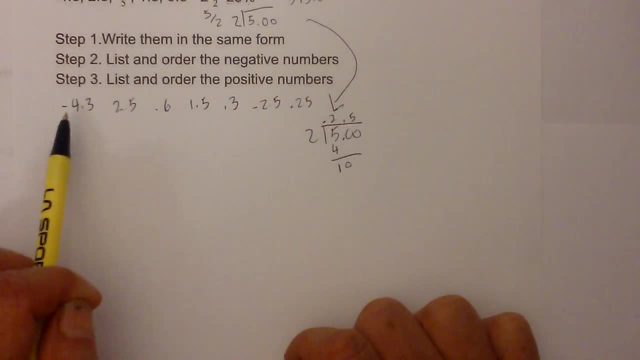 from least to greatest, because they're in the same form. So I'm going to start the negative number. I have negative four thirds. Remember, with negative numbers, the larger the number, the smaller it is. So I have negative four thirds. Now I have negative 2.5.. Okay, I'm going to put a check by this And now I'll start.